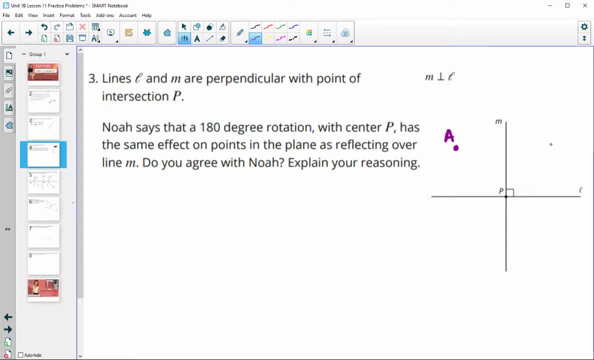 So, if we look at this as being point A, if we were to reflect this point over line M, it would end up over here, So this would be the image with a reflection. So then, if we think about a 180 degree rotation, 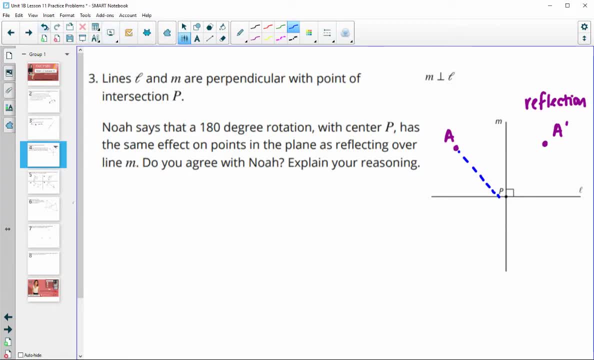 remember, when you do a 180 degree rotation, you kind of think about connecting it to that center point And they told us the center point is P, And then doing a 180 degree angle And that will tell you where the new point would land. 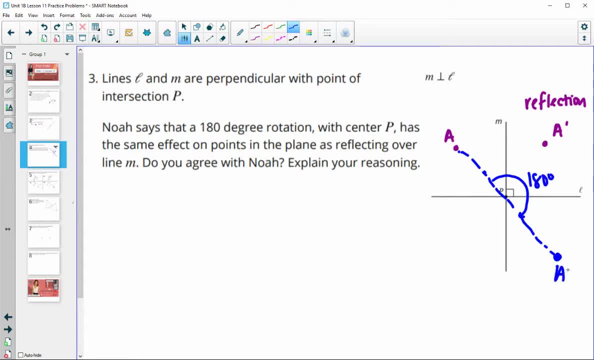 With a 180 degree angle, you're going to have a 180 degree rotation. So here would be the image of A after a rotation of 180 degrees. So they do not have the same impact because the reflection and the rotation of 180 are different. 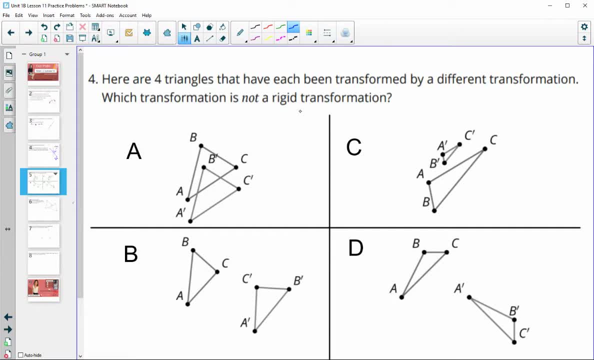 Number four gives us four triangles. Each has been transformed by a different transformation. Which one of these is not A rigid transformation? So not a rigid transformation. Remember, rigid transformation means that they stay the same size. So we are looking for two triangles that change sizes. 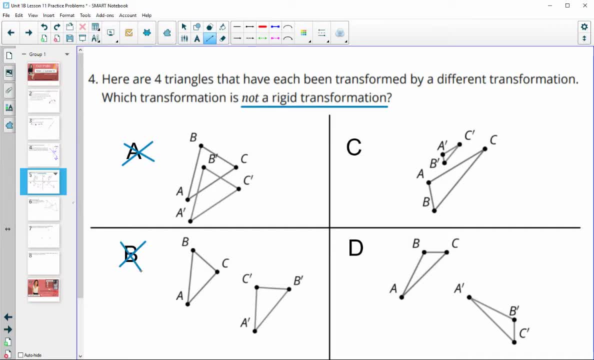 So the triangles in A stay the same, in B stay the same, in C they change. So that would be our answer. And in D they in fact don't change sizes again. So C is the one that is not a rigid transformation. 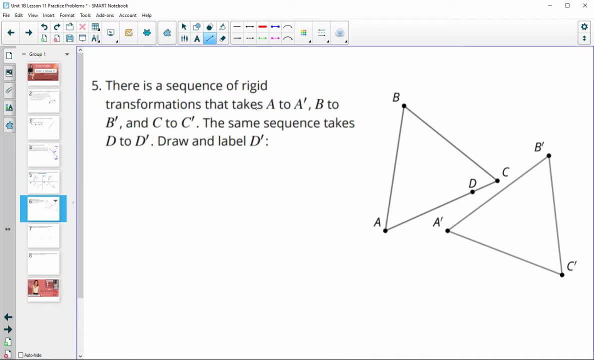 Number five: there's a sequence of rigid transformations that takes A to A prime, B to B prime and C to C prime. That same exact set of transformations is going to take D to D prime. So label where D prime would be. 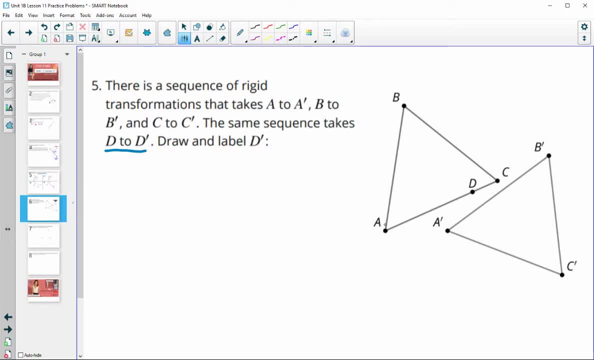 So D is going to have to be on the segment A prime, C prime, So it's on AC, So it's going to be on the image of AC And then it's pretty close to C, So it's going to stay. 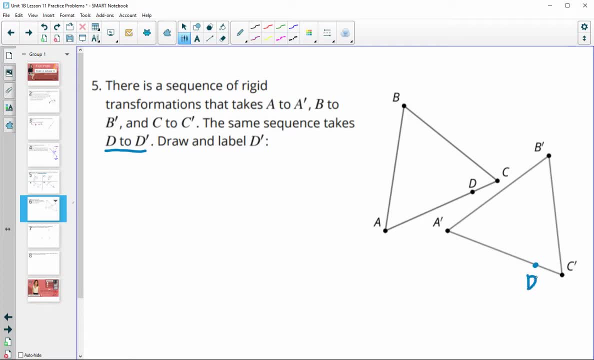 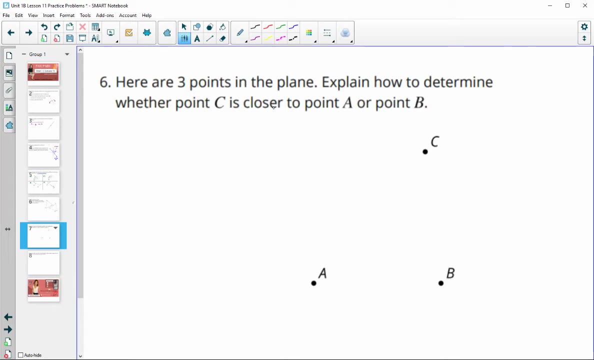 Pretty close. Well, the exact same length, But if you're sketching it you can just kind of guess. So the same distance from C prime as it was from C Number six. here are three points in the plane. Explain how you would determine whether C is closer to A or to B. 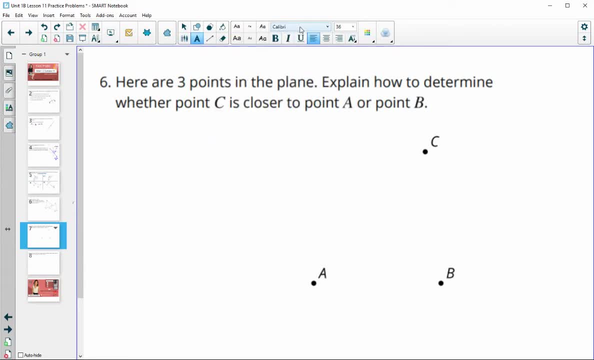 So if we were going to explain it, you could do I would construct the perpendicular bisector Of AB, since that will be all of the points that are the same distance from A and B. Then whichever side of the perpendicular bisector C is on, it is closer to that point. 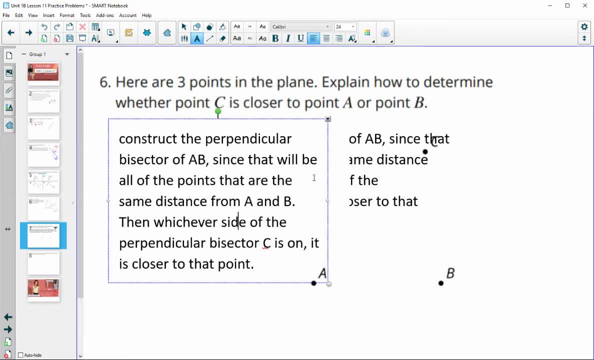 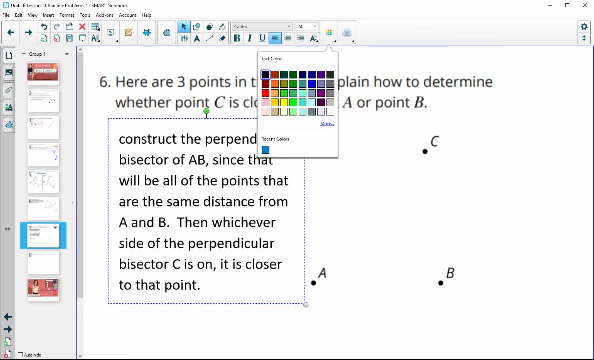 So let's, let me just move this a little bit, So if we just do that quick, so let me just construct the perpendicular bisector so I can tell you what we're looking at here. So I'm just going to do it with a circle instead of pulling out the compass. 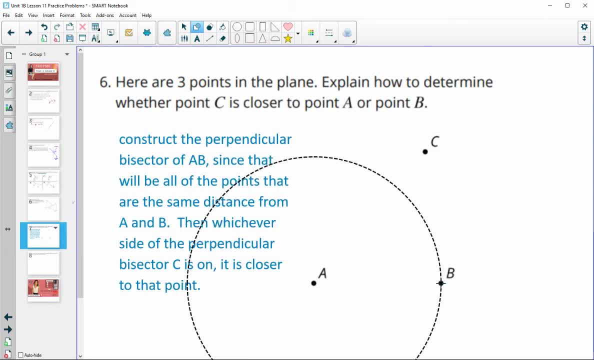 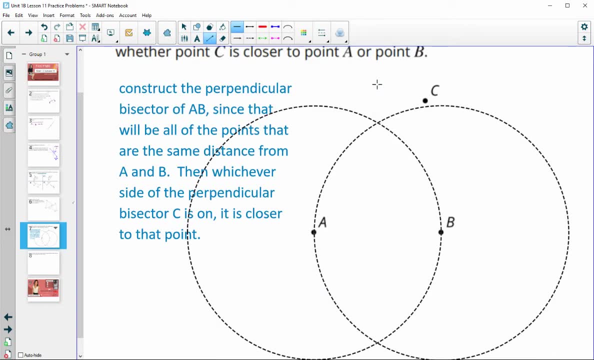 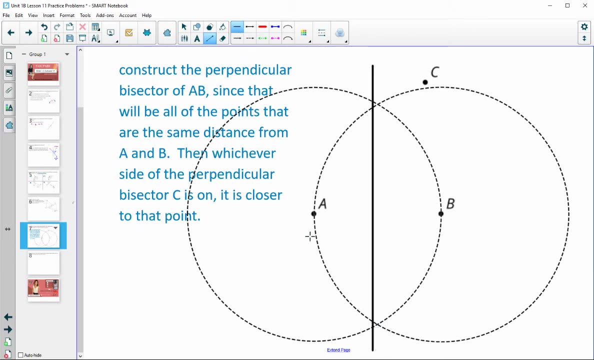 But so if I do a circle that goes through B and then that goes through A, this will give me my intersections for the perpendicular bisector. So here, whoops. So here would be the perpendicular bisector of segment AB. So the points along this line are equidistant. 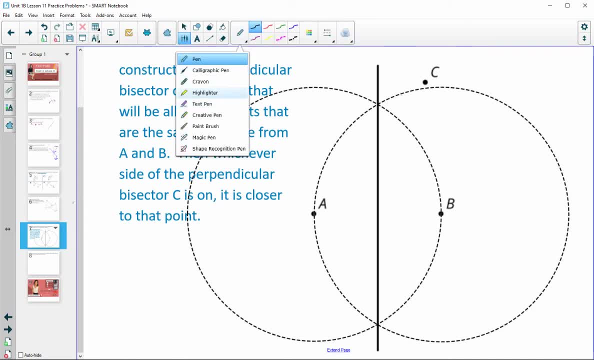 So any of the points in this side are going to be closer to B, So this side is- let me do that one more time. So this side is going to be closer to B. So C is on the B side. So C is closer to B. 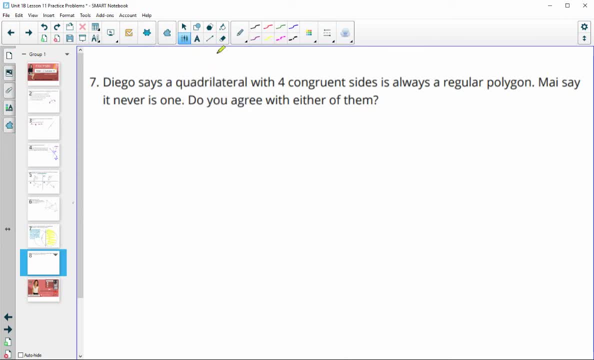 All right. number seven: Diego says a quadrilateral with four congruent sides is always a regular polygon. Mai says it is never one. Do you agree with either of them? So four congruent sides. So remember that regular means that it has equal sides and equal angles. 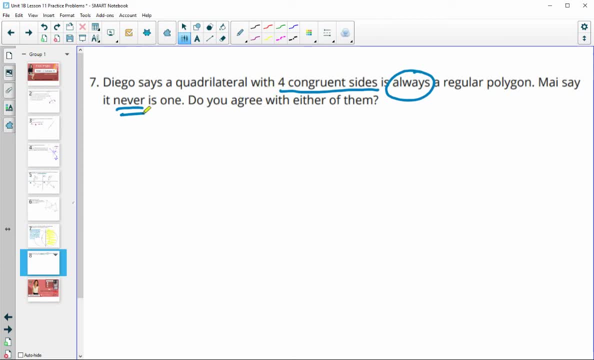 So basically, can we draw any that are regular, Then Mai would be wrong, And if we can draw any that don't have equal angles, then Diego would be wrong. So four equal sides is considered a rhombus, And so the rhombus- here's a rhombus- that does not have equal angles.